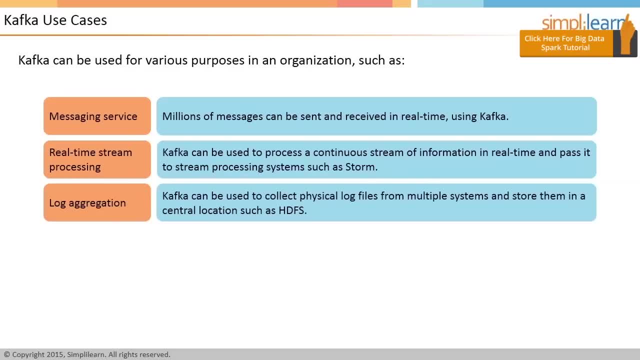 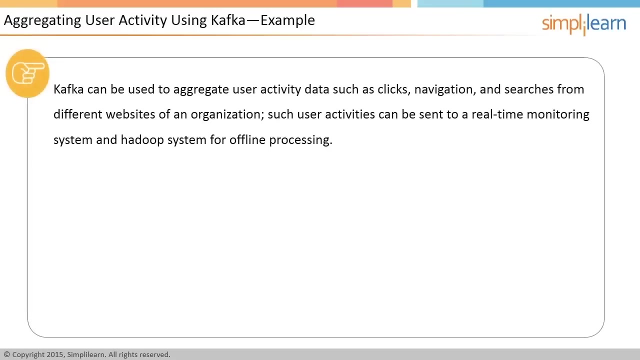 and to store it in essential location such as HDFS Commit log service. Kafka can be used as an external commit log for distributed systems. Event-sourcing, %, ordered sequence of events can be maintained through Kafka. Kafka can be used to aggregate user activity data, such as clicks, navigation and searches. 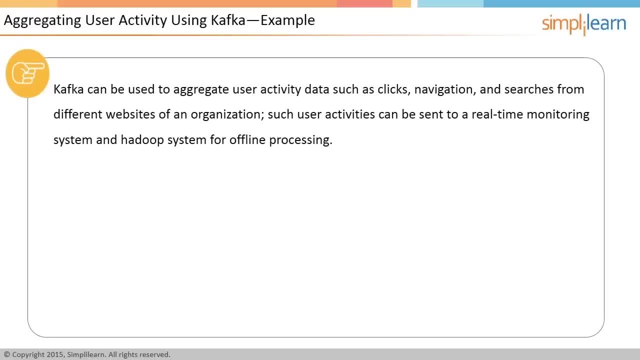 from different websites of an organization. Such users activities can be sent to a real-time monitoring system and Hadoop system for offline processing. An example is illustrated in the image. The information from customer facing portals are sent in real-time to the Kafka cluster. The Kafka cluster consists. 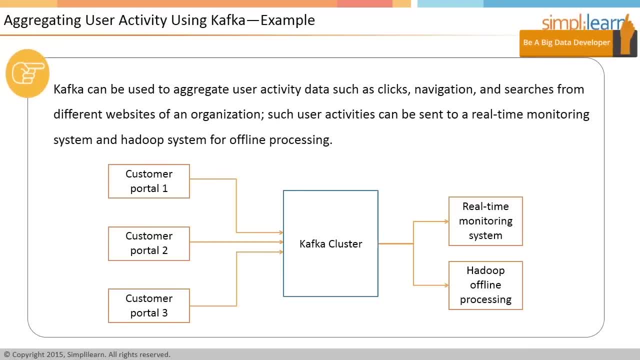 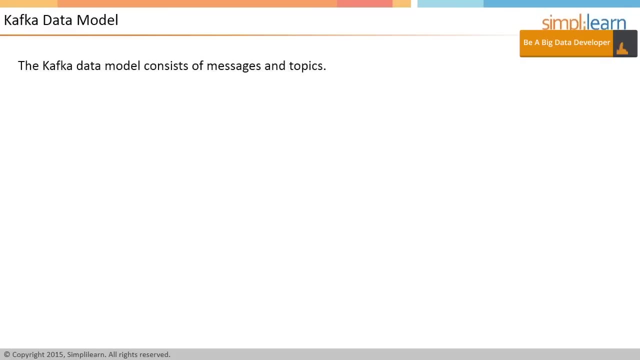 of one or more servers that process the messages in parallel. The information is sent to a real-time monitoring system to monitor the user clicks, navigation and searches. The information is also saved in a Hadoop system for offline processing. The Kafka data model consists of messages and topics. Messages: 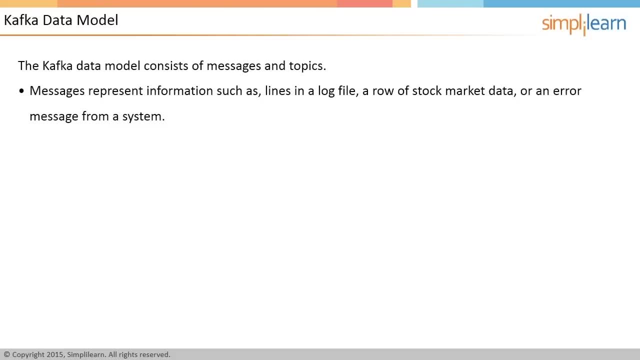 represent information such as lines in a log file, a row of stock market data or an error message from a system. Messages are grouped into categories called topics, for example log message and stock message. The processes that publish messages into a topic in Kafka are known. 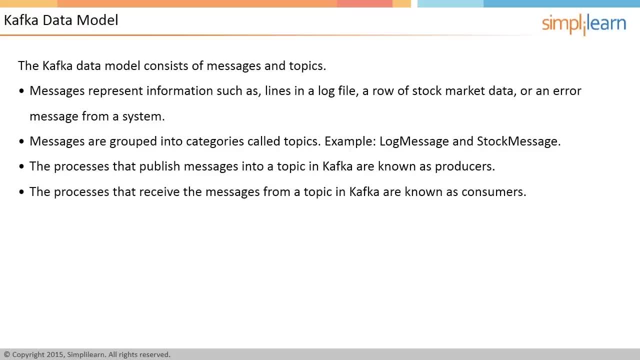 as producers. The processes that receive the messages from a topic in Kafka are known as consumers. The processes or servers within Kafka that process the messages are known as brokers. A Kafka cluster consists of a set of brokers that process the messages. The image illustrates the Kafka data model. It shows a Kafka cluster that consists of: 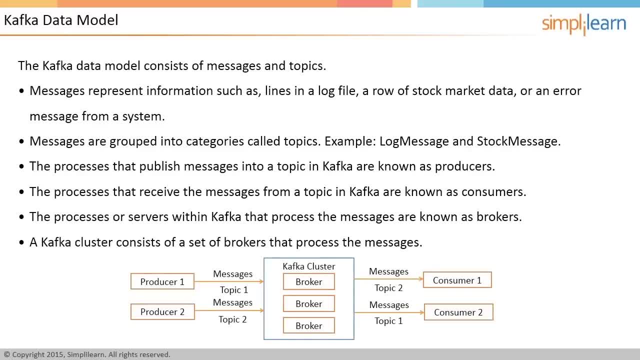 three brokers. There are two producers sending messages to the Kafka cluster and two consumers receiving the messages from the cluster. Producer 1 creates messages for topic 1, whereas producer 2 sends messages for topic 2.. These messages are processed by the three brokers in parallel and sent to the 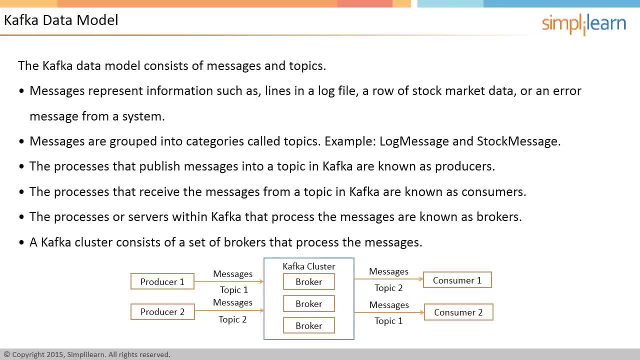 consumers. Consumer 1 is interested in topic 2, so it receives the messages for topic 2.. Similarly, consumer 2 is interested in topic 1, so it receives the messages for topic 1.. The brokers in the Kafka cluster handle the process of receiving. 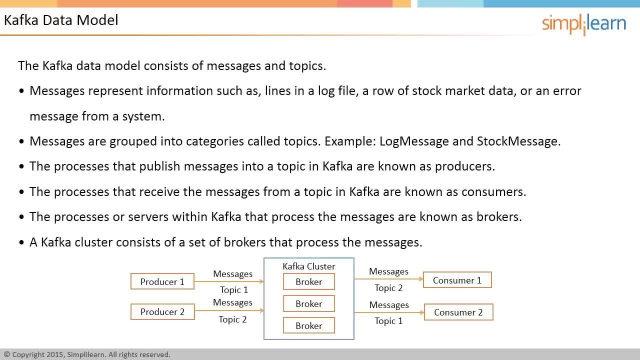 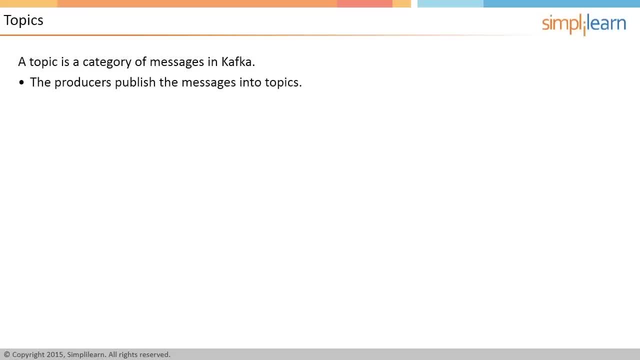 storing and forwarding the messages to the interested consumers. A topic is a category of messages in Kafka, The producers publish the messages into topics and the consumers read the messages from topics. A topic is divided into one or more partitions. A partition is also known as a. 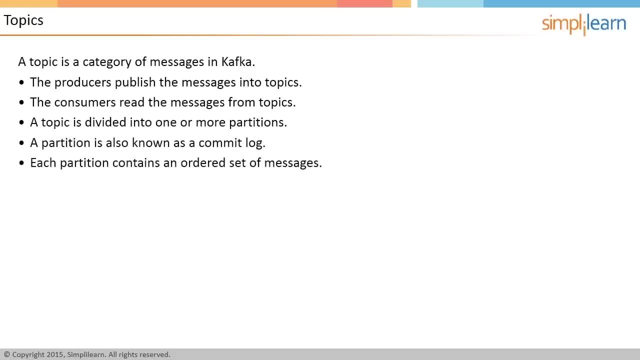 commit log. Each partition contains an ordered set of messages. Each message is identified by its offset in the partition. Messages are added at one end of the partition and consumed at the other. The image illustrates a topic simple that is divided into two partitions. The writes are completed at. 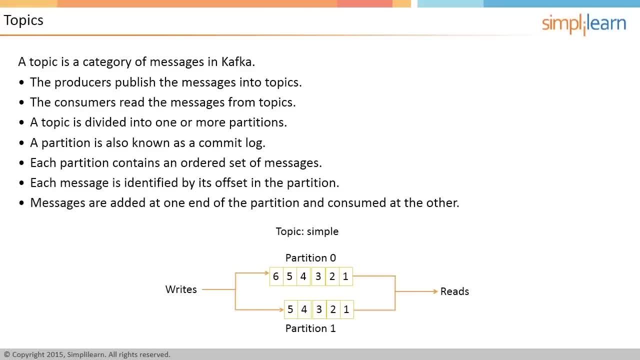 one end and the reads are completed at the other. It shows six messages in partition 0 and five messages in partition 1.. The offset of message 1 in partition 0 is 0, as it is the first message. The offset of message 6 in partition 0 is 5.. The messages are written in the order 1,, 2,, 3,. 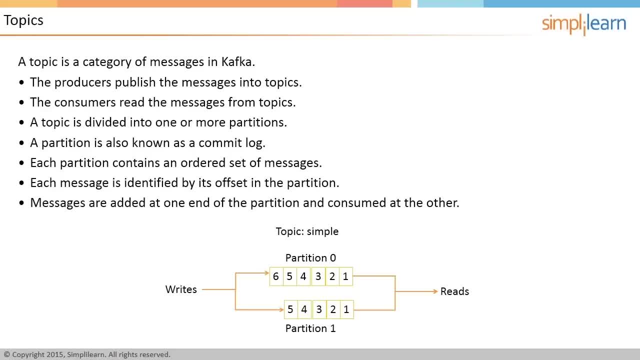 4,, 5, and 6,, whereas they are read in the same order as 1,, 2,, 3,, 4,, 5, and 6.. The next message in partition 0 will be message 7,, which will be written at: 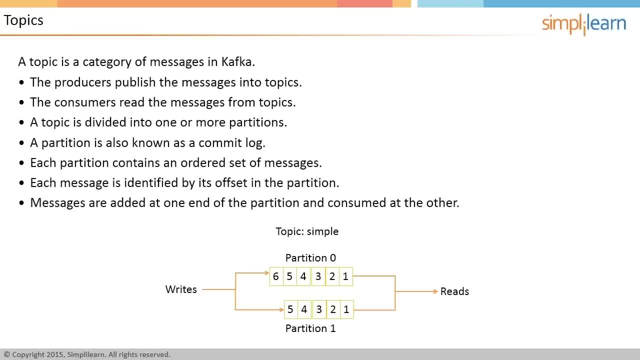 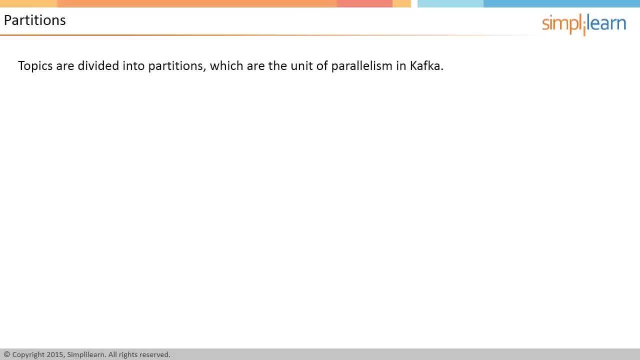 offset 6.. The next message for partition 1 will be message 6, which will be written at offset 5.. Topics are divided into partitions which are the unit of parallelism in Kafka. Partitions allow messages in a topic to be distributed to multiple servers or brokers. 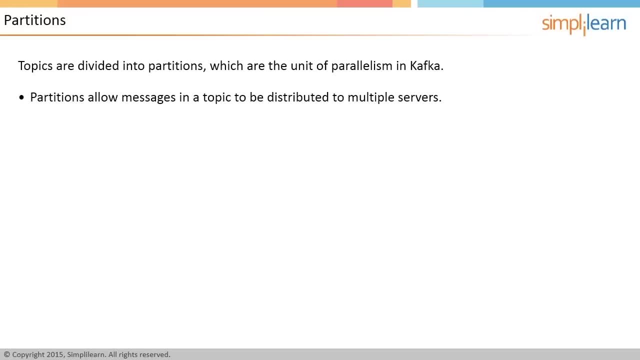 so that the messages in a topic can be processed in parallel. A topic can have any number of partitions. Each partition should fit in a single Kafka server. The number of partitions in a topic decide the parallelism of the topic. The image illustrates two partitions of a topic simple. 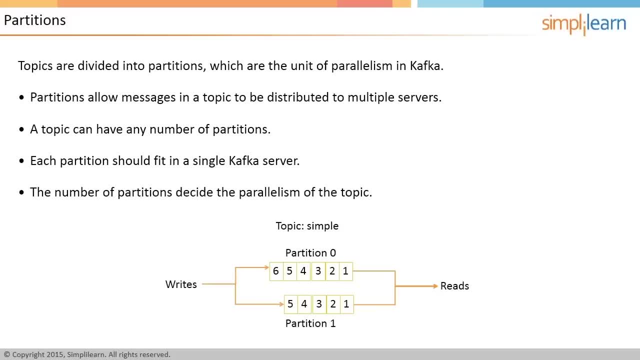 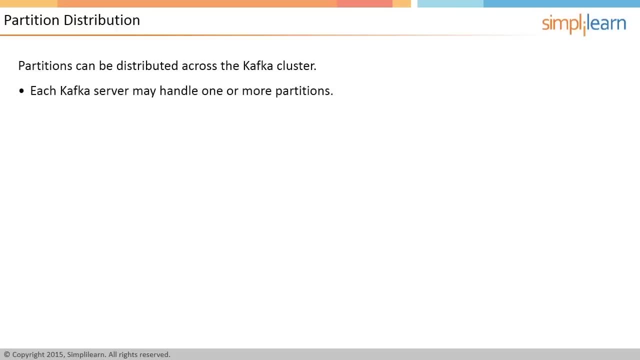 Partition 0 consists of 6 messages, whereas partition 1 consists of 5 messages. Partitions can be distributed across the Kafka cluster. Each Kafka server or broker may handle one or more partitions. A partition can be replicated across several servers for fault tolerance. 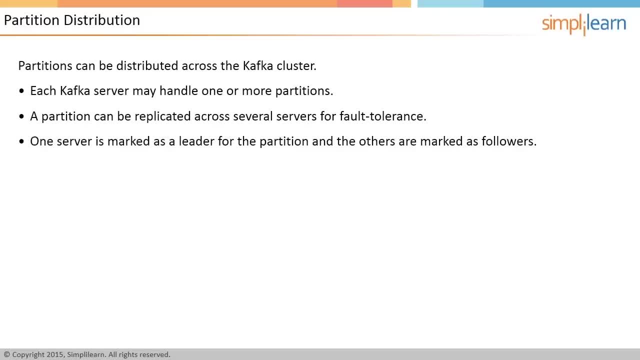 One server is marked as a leader for the partition And the others are marked as followers. The leader controls the read and write for the partition, whereas the followers replicate the data. If a leader fails, one of the followers automatically become the leader. 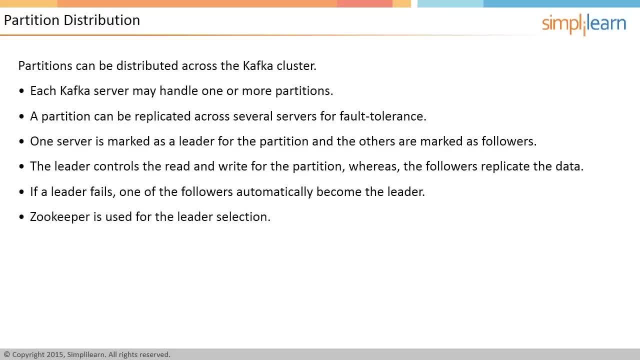 ZooKeeper is used for the leader selection, as explained in the previous lesson. The image illustrates the partition of a topic, simple. Here the partition 0 is assigned to server 1 and partition 1 is assigned to server 2.. These servers process the messages in parallel. 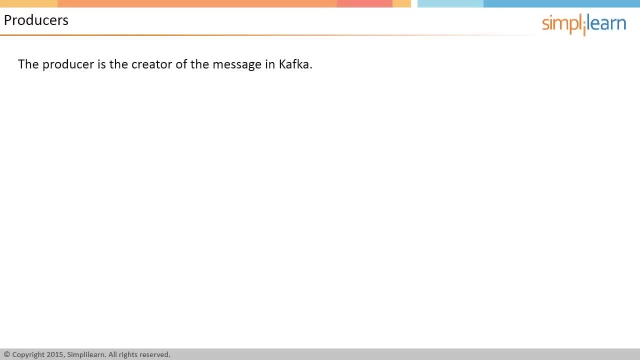 Partition 1 is assigned to server 2.. ARCHIVE: The producer is the creator of the message. in Kafka, Producers place the message to a particular topic and decide what partition to place the message into. For example, a producer may place a message into partition 0 of topic simple. 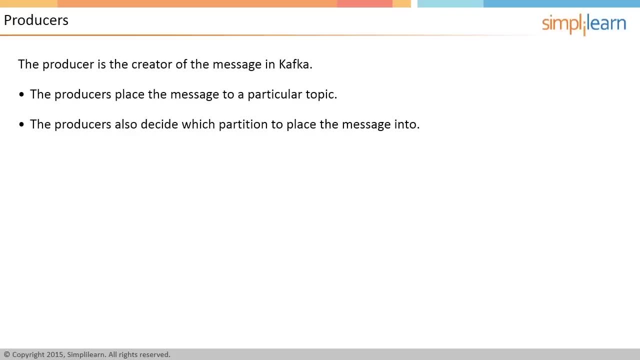 Another producer may place a message into partition 1 of topic. simple Topics should already exist before a message is placed by the producer. Messages are added at one end of the partition by Kafka Kafka. The image illustrates a producer that creates three messages and sends them to different. 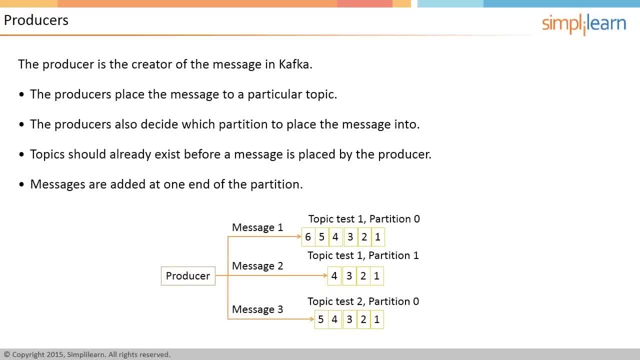 topics and partitions in Kafka. Message 1 is sent to partition 0 of topic test 1,, message 2 is sent to partition 1 of topic test 1, and message 3 is sent to partition 0 of topic test 2.. 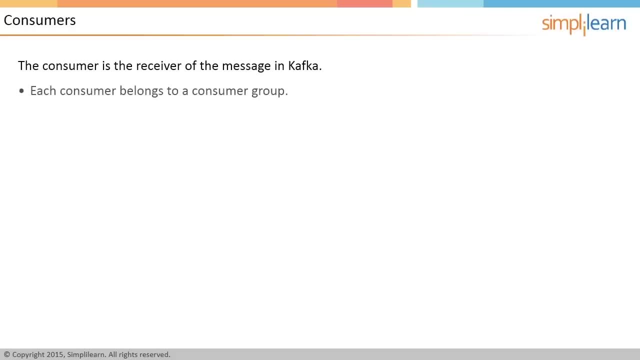 The consumer is the receiver of the message in Kafka. Each consumer belongs to a consumer group. A consumer group may have one or more consumers. The consumers specify what topics they want to listen to. A message is sent to all the consumers in a consumer group. 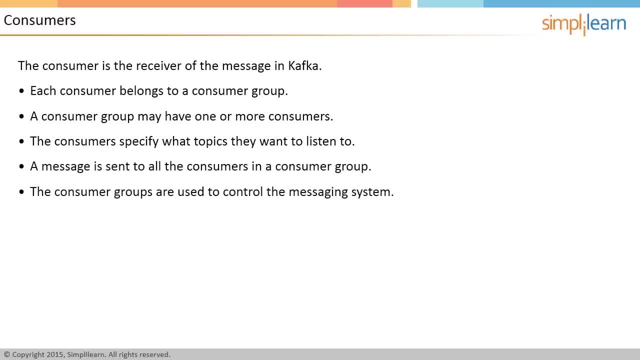 The consumer groups are used to control the messaging system. The image illustrates the three consumer groups. They are consumer group 1, consumer group 2, and consumer group 3.. The consumer group 1 consists of three consumers called consumer 1, consumer 2, and consumer. 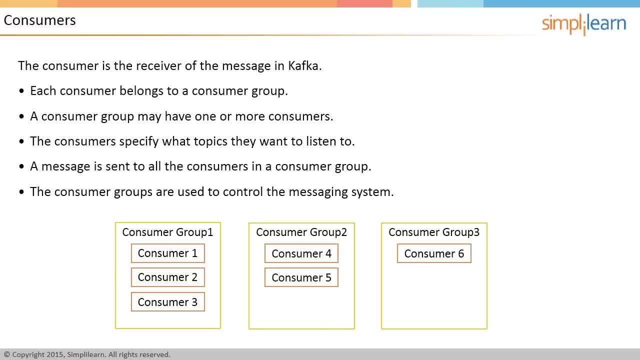 3.. The consumer group 2 consists of two consumers called consumer 3.. Consumer group 4 and consumer 5.. The consumer group 3 consists of a single consumer called consumer 6.. Kafka architecture consists of brokers that take messages from the producers and add to. 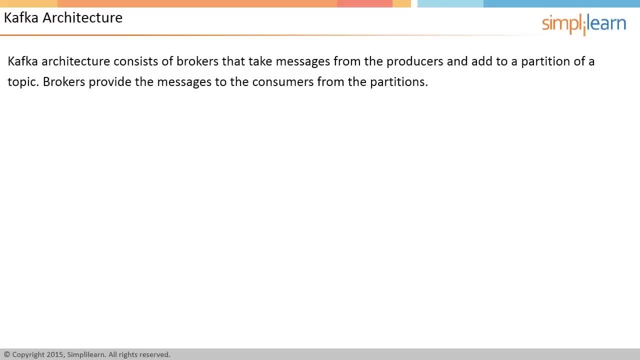 a partition of a topic. Brokers provide the messages to the consumers from the partitions. The producers create the messages and send them to a particular topic and a partition of a Kafka cluster. A topic is divided into multiple partitions. The messages are added to the partitions at one end and consumed in the same order. 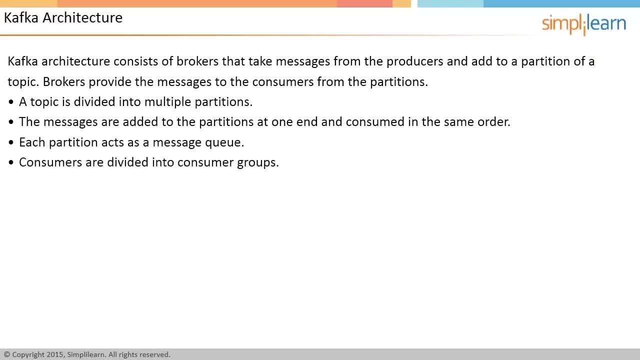 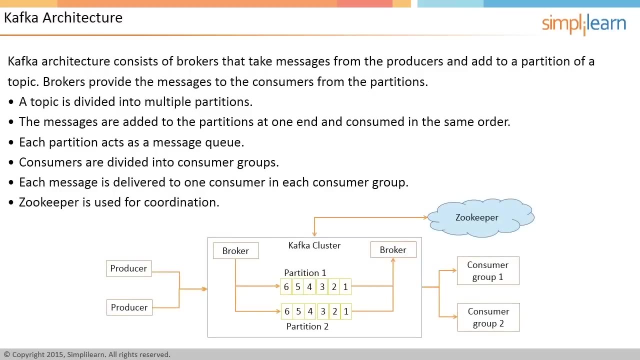 Each partition acts as a message queue. Consumers are divided into consumer groups. Each message is delivered to one consumer in each consumer group. Zookeeper is used for coordination among the Kafka brokers. The image illustrates the Kafka architecture that consists of two partitions called partition. 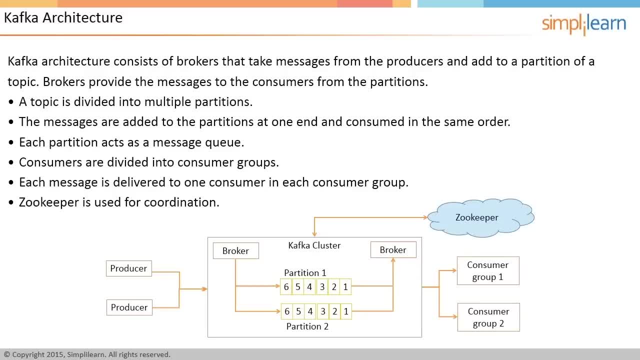 1 and partition 2.. The two producers are sending messages to the two brokers in the cluster. The two producers are sending messages to the two brokers in the cluster. The brokers add the messages to the partitions and the messages are taken from the partitions. 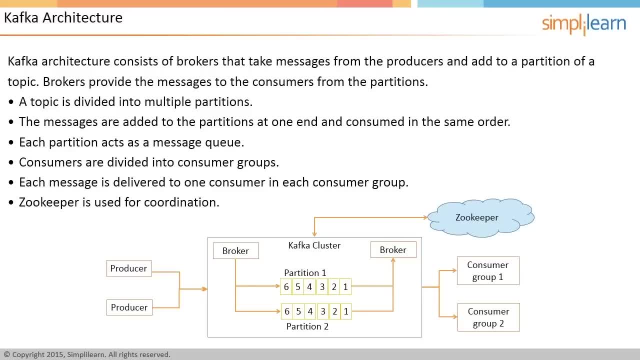 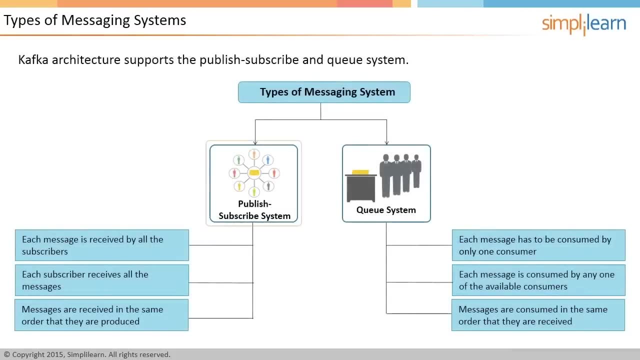 in the same order as insertion, The messages are sent to two consumer groups. The image also illustrates that the Kafka cluster, or brokers, interact with Zookeeper for distributed coordination. Kafka architecture supports two types of messaging systems, known as Publish-Subscribe and Queue System. 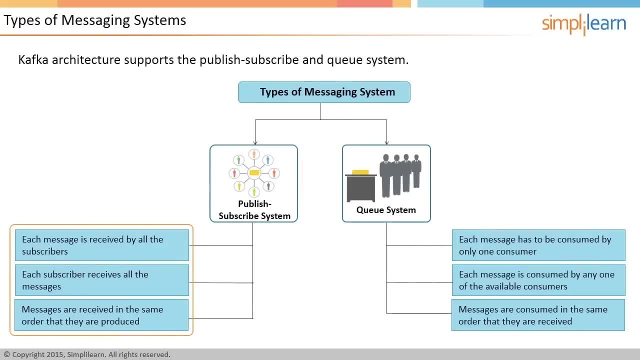 The Publish-Subscribe system is also called Pub-Sub. In this system, one system broadcasts the messages and the consumers subscribe to receive the messages. Each message is received by all the subscribers. so if there are 100 messages published, each subscriber receives all the 100 messages in the same order that they are produced. 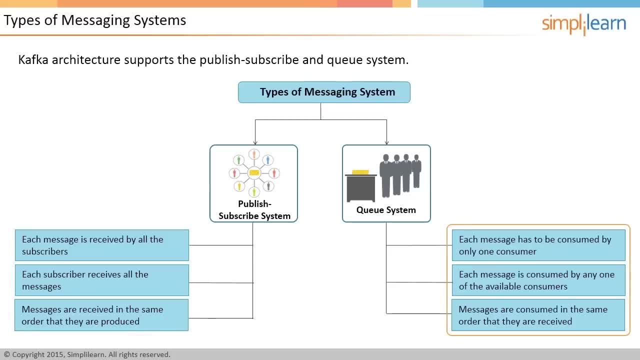 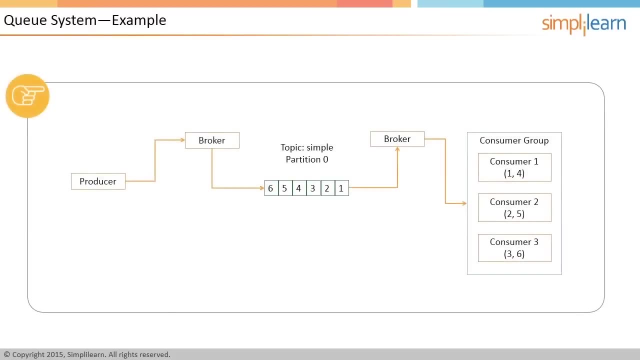 In the Queue system, each message has to be consumed by only one consumer. If there are multiple consumers, each message is consumed by any one of the available consumers in the same order that they are received. The image illustrates the implementation of a Queue system. 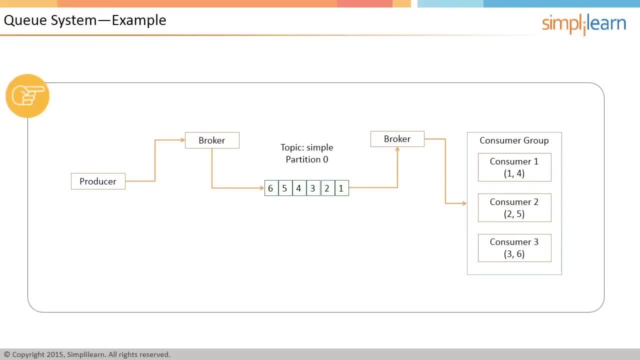 Consumer 1,, Consumer 2, and Consumer 3 belong to the same consumer group. So out of the 6 messages, 2 messages are received by Consumer 1,, 2 messages by Consumer 2, and 2 messages by Consumer 3.. 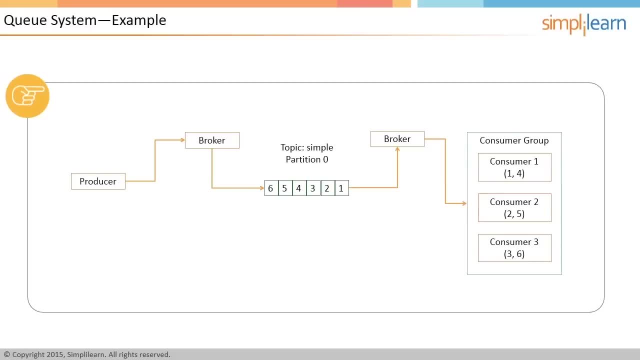 Note that the messages are received in the same order that they are produced, So Consumer 1 receives message 1, Consumer 2 receives message 2, and Consumer 3 receives message 3.. After this, Consumer 1 receives message 4, Consumer 2 receives message 5, and Consumer 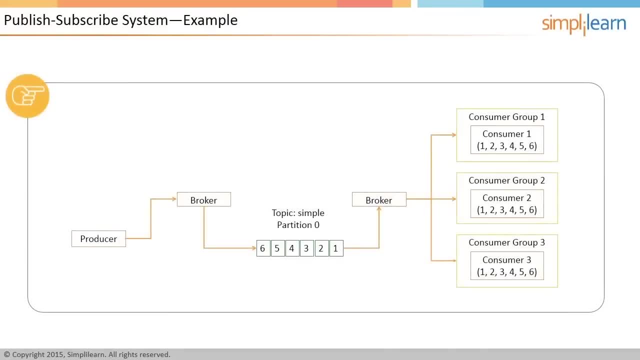 3 receives message 6.. The image illustrates the implementation of a Pub-Subscribe system. Consumer 1,, Consumer 2, and Consumer 3 belong to 3 separate consumer groups, So all the 6 messages are sent to all the 3 consumer groups, called Consumer Group 1,. 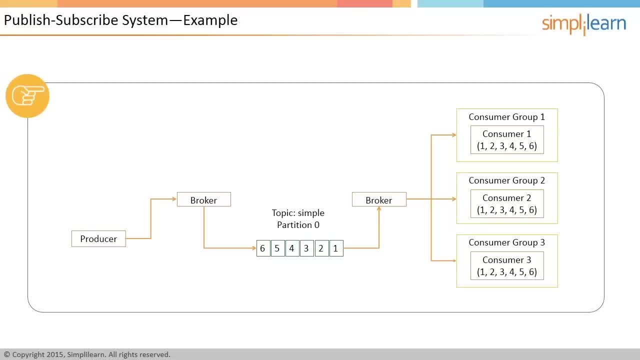 Consumer Group 2, and Consumer Group 3.. Since there is only one consumer in Consumer Group 1, the image illustrates the implementation of a Pub-Subscribe system. So Consumer 1 receives all the 6 messages in the order: 1,, 2,, 3,, 4,, 5, and 6.. 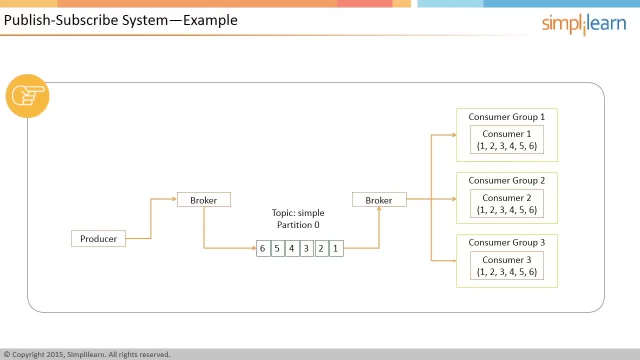 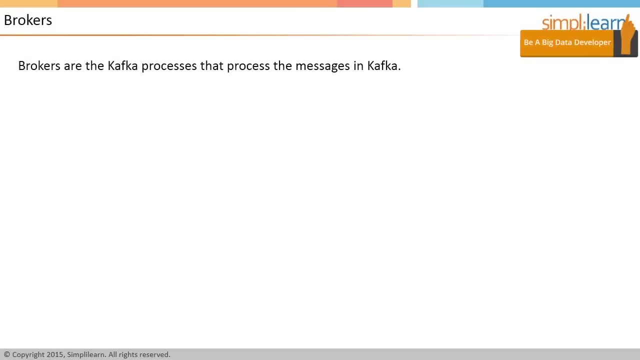 Similarly, Consumer 2 and Consumer 3 also receive all the 6 messages in the same order. Brokers are the Kafka processes that process the messages in Kafka. Each machine in the cluster can run one broker. The brokers coordinate among each other using ZooKeeper. 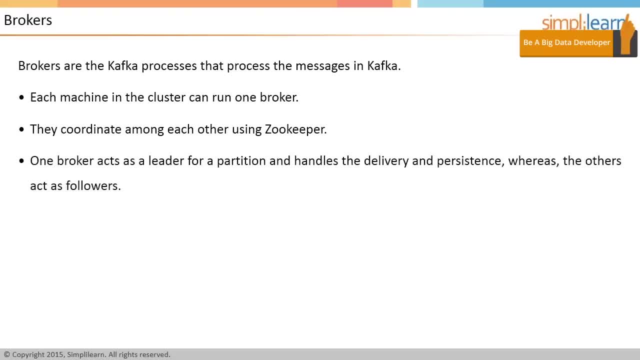 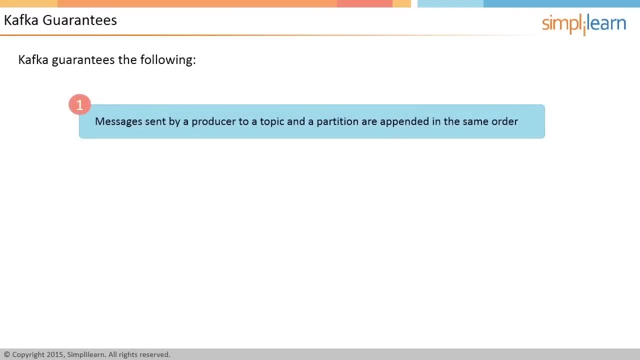 One broker acts as a leader for a partition and handles the delivery and persistence, whereas the others act as followers. Brokers receive the message from the producer and send it to the consumer groups. Kafka guarantees the following Guarantee: 1. Messages sent by a producer to a topic and a partition are appended in the same order. 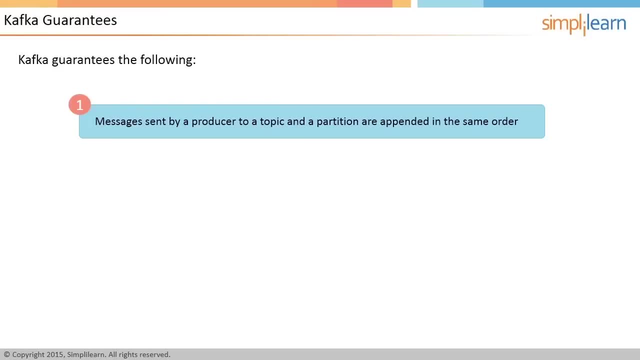 This ensures that the messages produced earlier do not get ahead of the messages produced later. The time order is maintained very strictly. Guarantee 2. A consumer instance gets the messages in the same order as the producer. The time order is maintained very strictly. 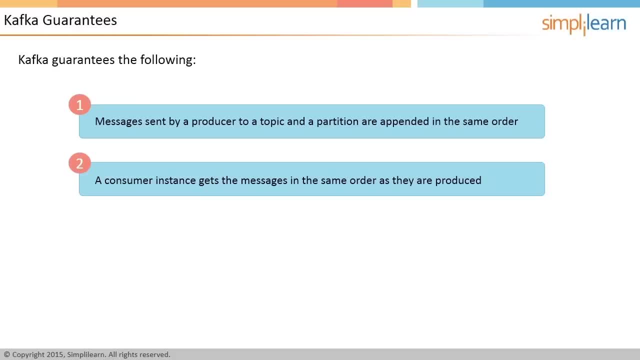 Guarantee 2.. If the messages are produced in the order 1,, 2,, 3,, 4,, 5,, 6,, they will be received in the order 1,, 2,, 3,, 4,, 5, and 6.. 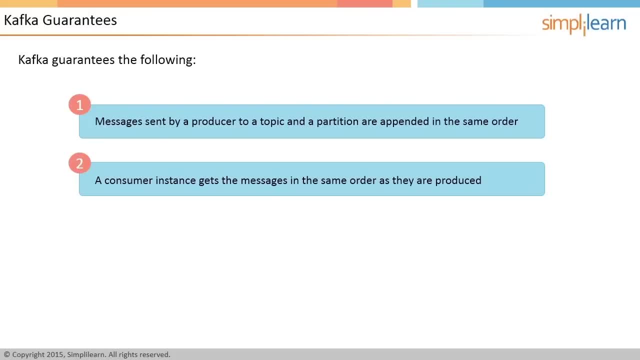 This is important in messaging systems as the dependency is on the time order of messages. Guarantee 3. A topic with replication factor N tolerates up to N-1 server failures, For example, when the replication factor is specified as 3.. There will be no loss of messages even if two machines fail. 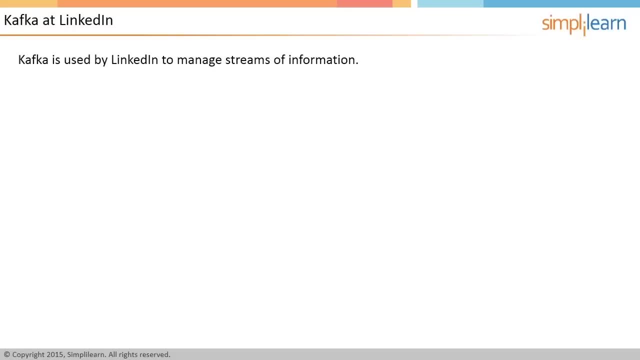 Guarantee 4.. LinkedIn, or the website wwwlinkedincom, is the largest network of professionals and is the originator of Kafka. Kafka is used by LinkedIn to manage streams of information. Some of the uses of Kafka at LinkedIn are as follows: Guarantee 5.. 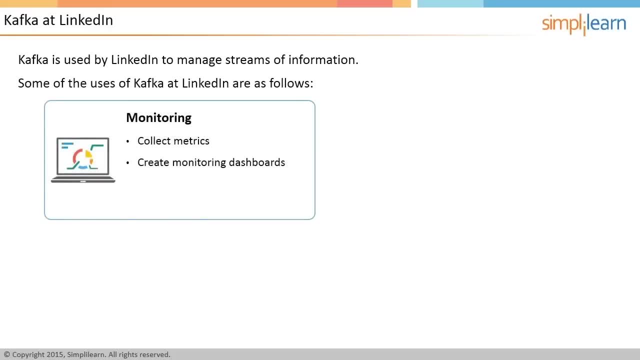 Monitoring: Kafka is used to collect metrics from various systems and to create monitoring dashboards. Guarantee 6. Kafka is used as message queues for content feeds and as publish-subscribe system for searches. Guarantee 7. Analytics: Kafka is used to collect page views and clicks from customer-facing websites and to store. 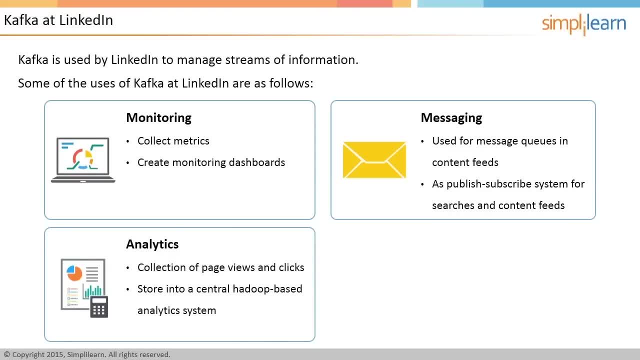 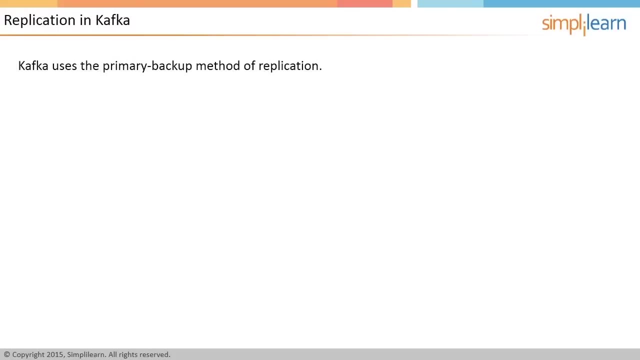 the information into a central Hadoop-based analytics system. Guarantee 8. A building block for distributed applications. Kafka is used as a building block for distributed applications and for building distributed databases and distributed log systems. Guarantee 9. Replication: Kafka uses the primary backup method of replication. 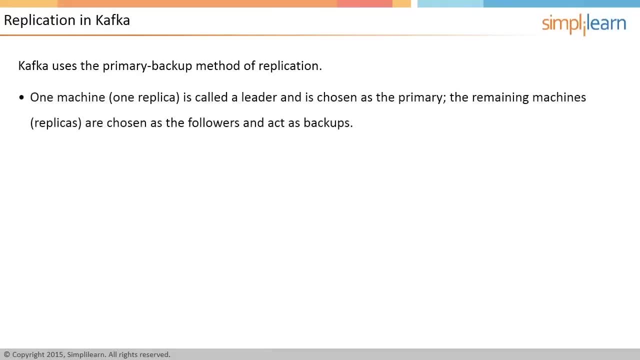 In primary backup method, one machine or one replica is called a leader and is chosen as the primary. The remaining machines or replicas are chosen as the followers and act as backups. The leader propagates the writes to the followers and waits until the writes are completed on. 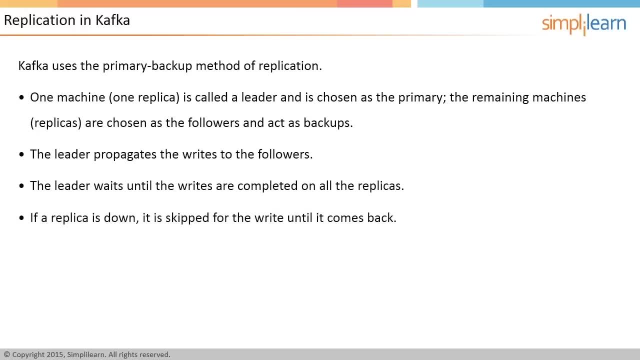 all the replicas. If a replica is down, it is skipped for the write. However, Kafka will write a copy to the machine once it is back. Guarantee 10.. If the leader fails, one of the followers will be chosen as the new leader. 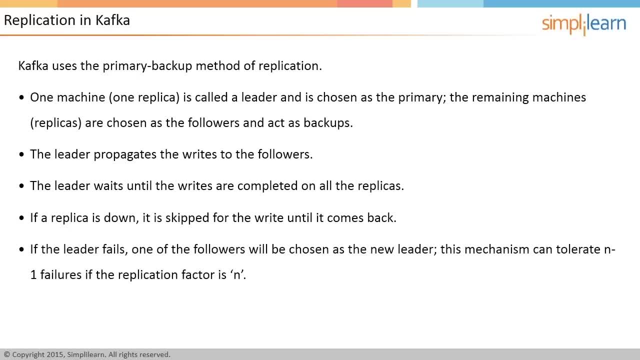 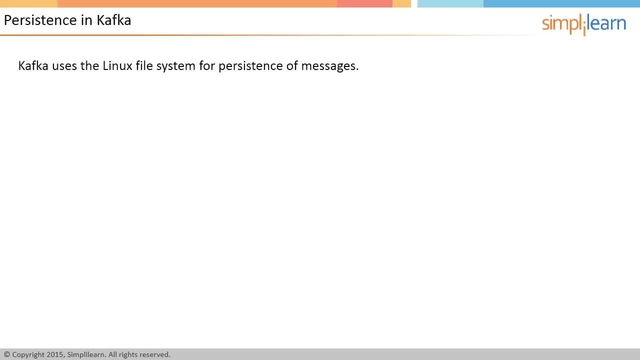 This mechanism can tolerate N-1 failures if the replication factor is N, which can be specified at the topic level. Persistence means a message can be delivered even if the machine that handles the message fails. Kafka uses the Linux file system for persistence of messages. 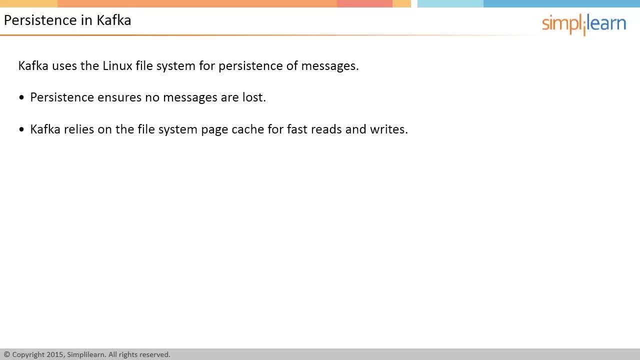 Persistence ensures no messages are lost. Kafka relies on the file system page cache for fast reads and writes Guarantee 11.. All the data is immediately written to a file in a file system so that they can be recovered even if the machine fails. Messages are grouped as message sets for more efficient writes. 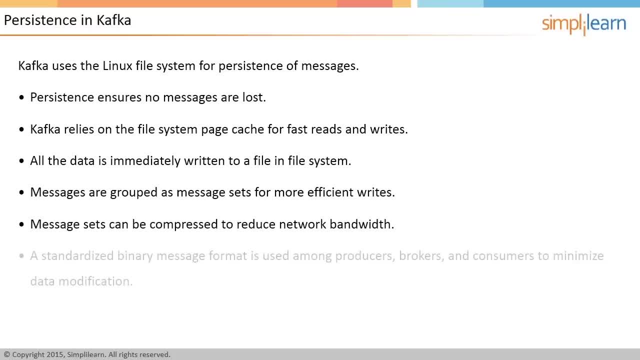 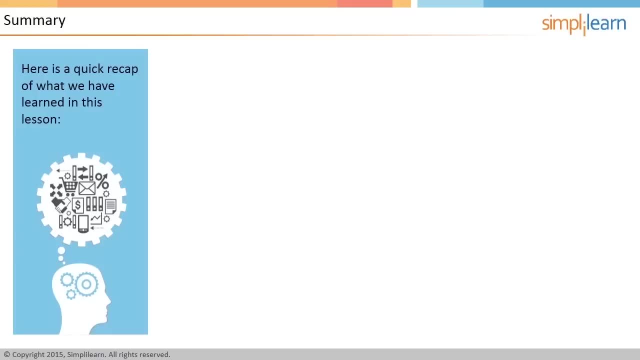 Message sets can be compressed to reduce network bandwidth. A standardized binary message format is used among producers, brokers and consumers to minimize data modification. Here is a quick recap of what we have learned in this lesson 1. Kafka is a high-performance real-time messaging system.